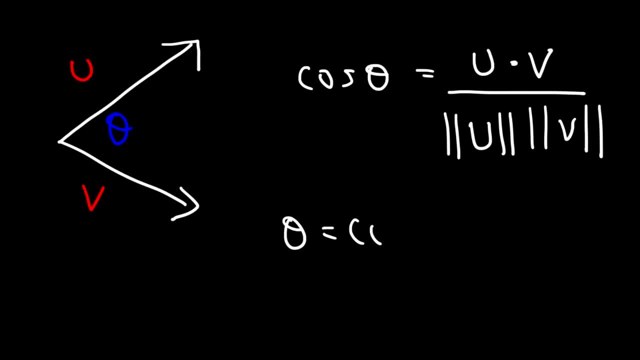 Now, to actually calculate the angle, you need to use the arc cosine function of the value that you get- Okay With the fraction on the right side. So once you get an answer, you need to take the arc cosine of that answer and that's going to give you the angle. 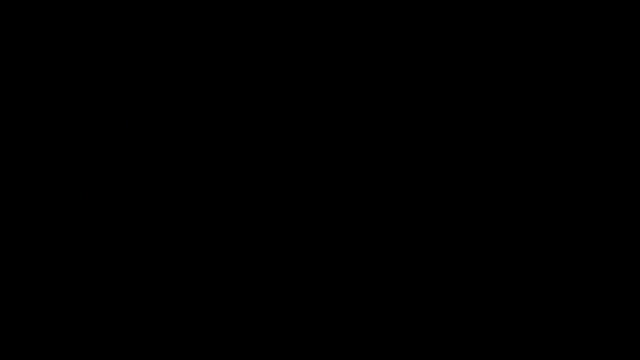 But let's go over some examples showing how we can do this. So let's say that vector u is equal to negative 2 comma 5 and vector v is equal to 4 comma 3.. So, given these two vectors, go ahead and calculate the angle between those two vectors. 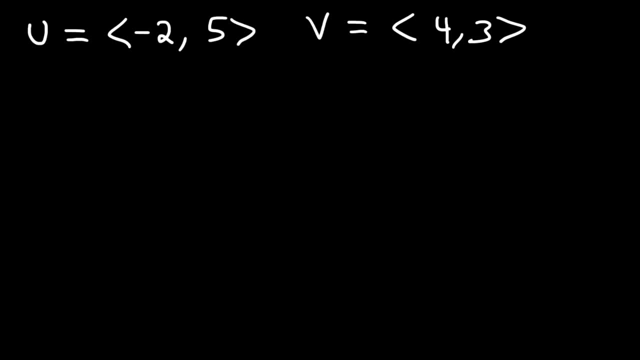 So the first thing I'm going to do is calculate the dot product of the two vectors u and v. So we need to multiply the x components of vector u and v, So it's negative 2 times 4.. And then we need to multiply the y components of those two vectors. 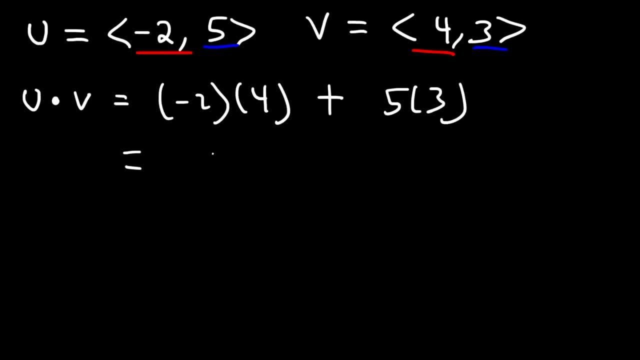 So we have 5 times 3.. And negative: 2 times 4 is negative 8.. 5 times 3 is 15.. And so this adds up to positive 7.. Now our next step is to calculate the magnitude of vector u. 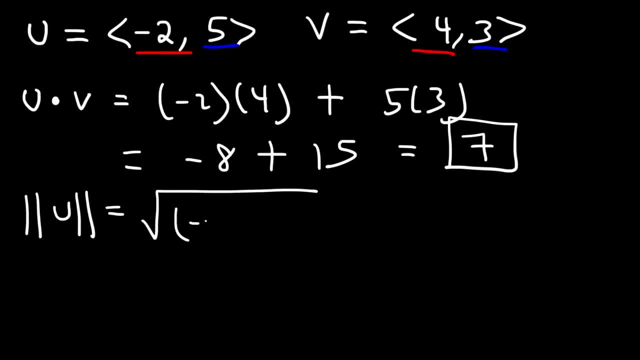 And it's going to be the square root of the square of the exponent and the square of the y component of vector u. So this is the x component of vector u and this is the y component. Negative 2 squared is 4. And 5 times 5 is 25.. 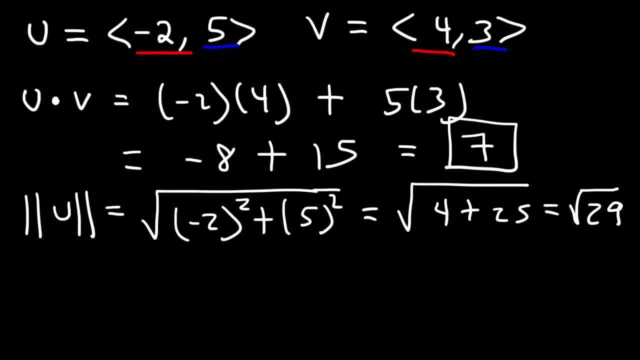 And so we get the square root of 29.. Now the next thing we need to do is calculate the magnitude of vector v, using the same process but with different numbers. So it's going to be the square root of 4 squared plus 3 squared. 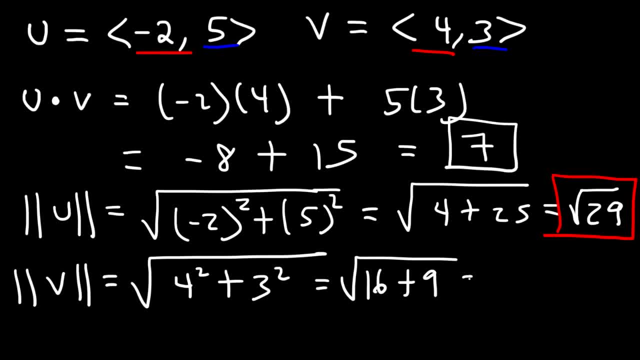 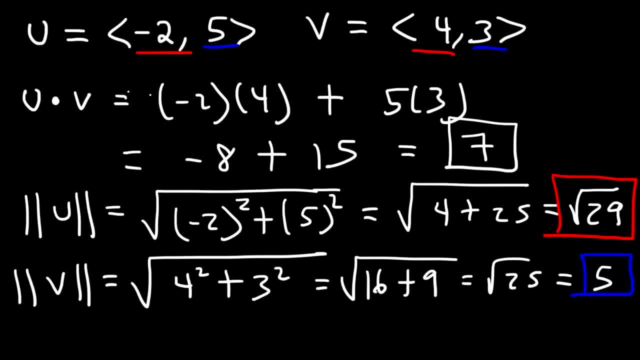 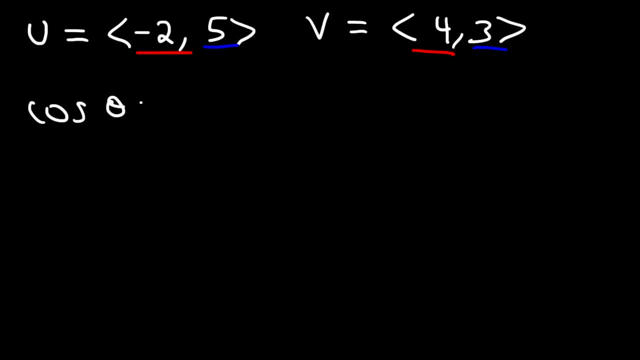 And that's equal to 4.. Now let's use that formula that we had in the beginning. So cosine theta is equal to the dot product of u and v divided by the magnitude of vector u times the magnitude of vector v. And so we saw that the dot product of u and v 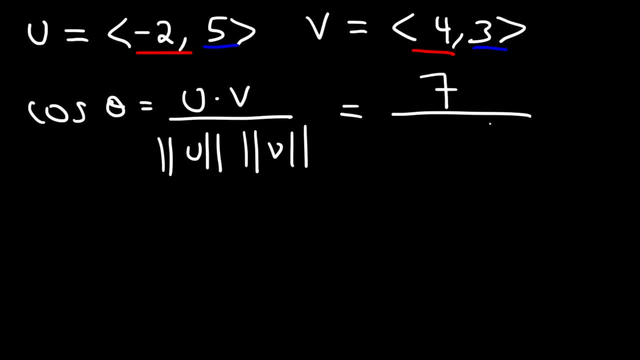 was 7,, the magnitude of vector u was the square root of 29, and for v it was just positive 5.. So what we need to do is calculate the angle theta by typing this in our calculator. So type in arc: cosine of 7 divided by 5 square root 29.. We 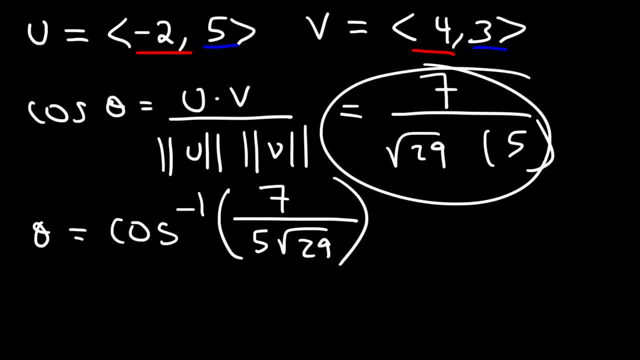 really don't need to rationalize this denominator. because we don't need to rationalize this denominator because we don't need to. It's not going to change your final answer Now it's going to help if you put this in parentheses for those of you who may. 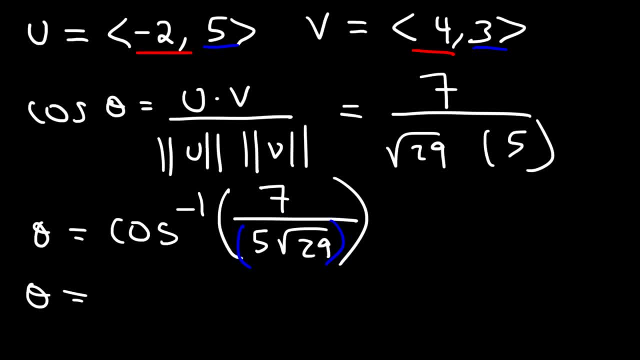 not be getting the right answer after trying this problem. So you should get 74.93 degrees. So that's the answer for this problem. If you want to, you can put your calculator in radian mode and get the angle in radians, But that's how you can find the. 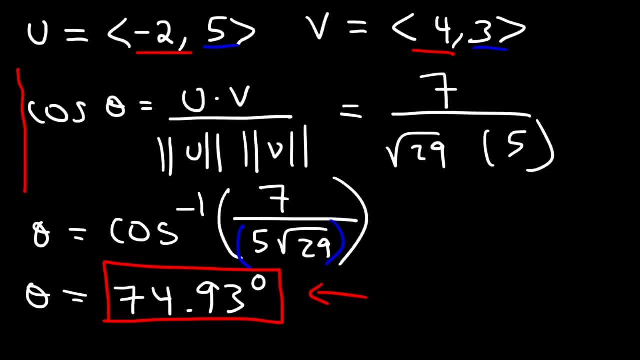 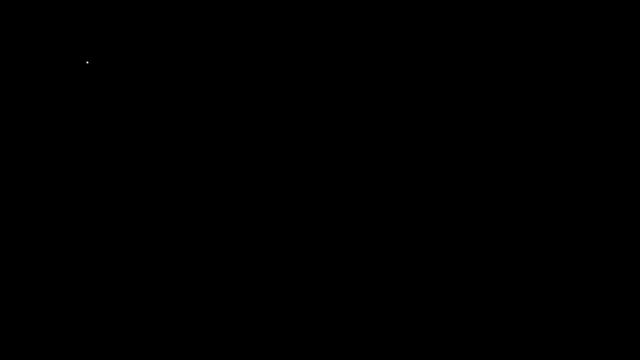 angle between two vectors simply by using this formula. Now let's try another example using three-dimensional vectors. So let's say we have vector u, which is 3 comma negative 4 comma 5.. And vector v, which is 2 comma 7 comma negative 3. Go ahead and calculate the. 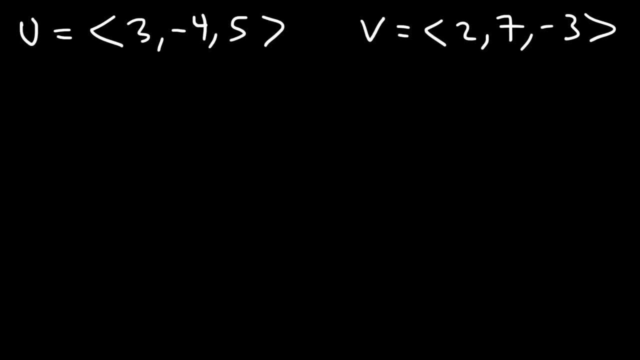 angle between those two vectors. So let's follow the same process. Let's begin by calculating the dot product of those two vectors. So let's multiply the x components together and that's going to be 3 times 2.. And then let's multiply the. 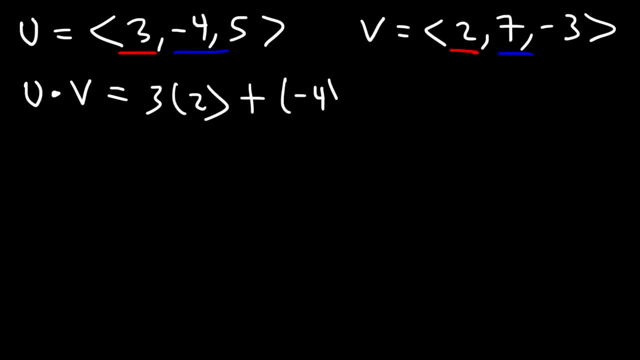 y components together, So that's negative 4 times 7.. And then finally multiply the z components And that's going to be 5 times negative: 3.. 3 times 2 is 6.. Negative 4 times 7, that's. 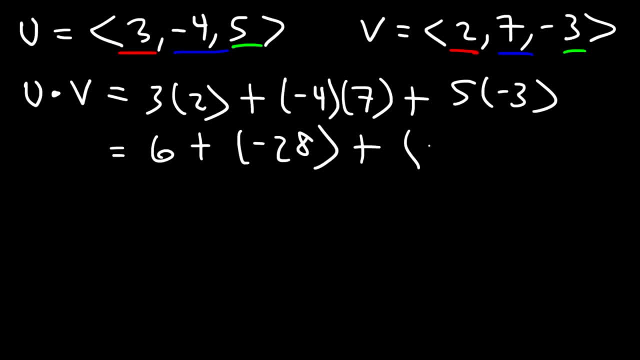 negative 28.. And 5 times negative 3,, that's negative 15.. Now 6 minus 28 is negative 22.. And negative 22 minus 15 is negative 37. So I'm just going to do that, I'm just going to write it over here: The dot product of the two vectors is negative. 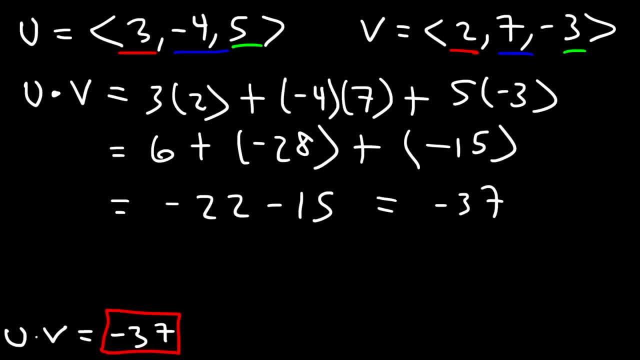 37. So we'll keep that for reference. Now our next step is to calculate the magnitude of vector u, And for a three-dimensional vector, it's going to be the square root of the square of the x component plus the square of the 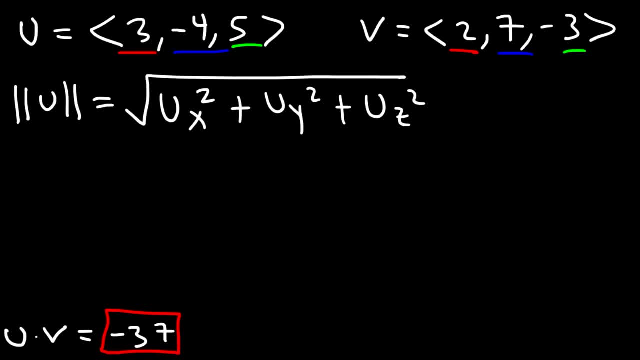 y component plus the square of the z component. So it's going to be the square root of 3 squared plus negative 4 squared plus 5 squared. Now, 3 squared is 9.. Negative 4 squared is 16.. 5 squared is 25.. 16 plus 9 is 25 plus. 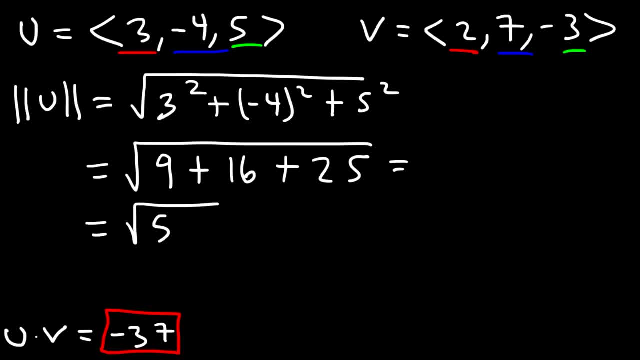 another 25.. That gives us 50.. And 50 is 25 times 25.. And the square root of 25 is 5.. So thus we have: the magnitude of u is equal to 5, square root 2.. Now let's calculate the magnitude of vector v. 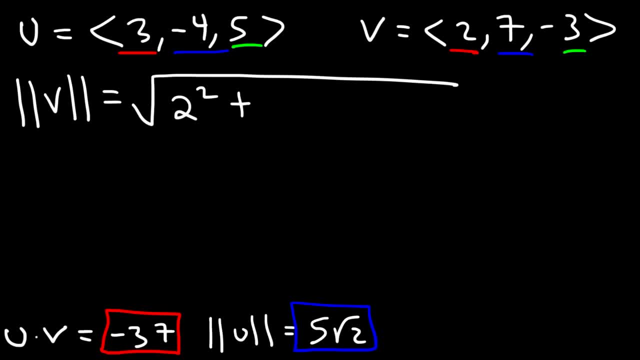 So, using the same formula, it's going to be the square root of 2 squared plus 7 squared plus negative 3 squared, 2 squared is 4.. 7 times 7 is 49.. Negative- 3 times negative, 3 is 9.. 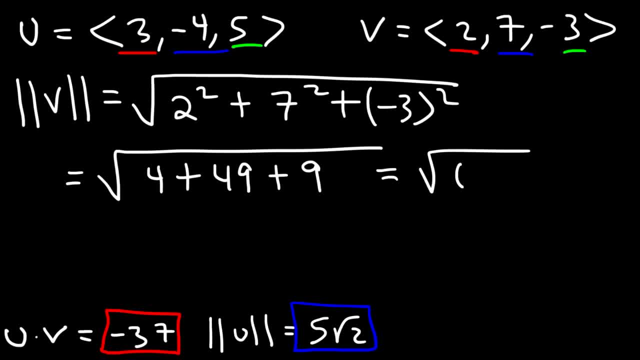 Now 4 plus 49,, that's 53, plus 9,, that gives us 62,, which I'm going to leave it like that. So now let's use the formula. We could jump to this version of the formula. The angle is equal to the arc cosine.